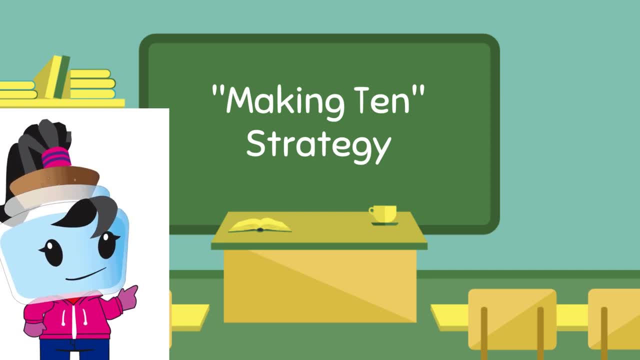 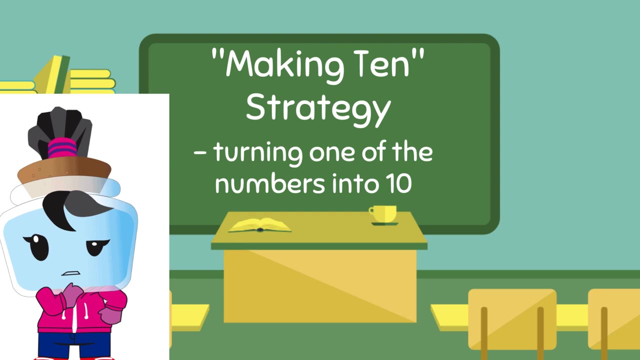 is the making 10 strategy. You might be asking: how can 10? help me add. This is where the making 10 strategy comes in. This strategy is when you try to turn one of the numbers in an addition problem into 10.. Let's try solving this. 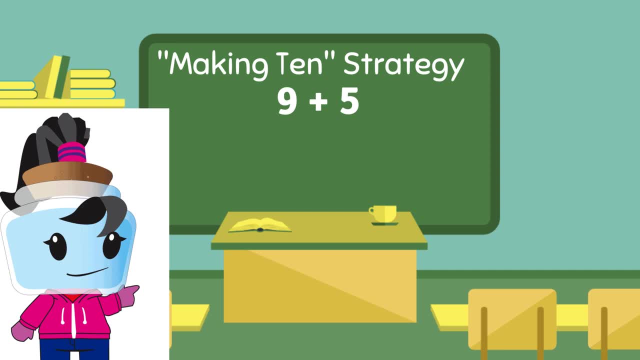 9 plus 5.. Try adding a value to 9. that will make it 10.. Do you know how much we'll need to add to 9 to make it 10?? That's correct, If we add 1 to 9, we get a 10.. But where do we get the 1 from? 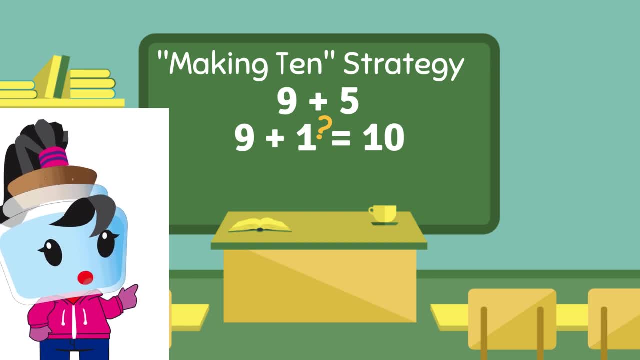 That's right- From the 5.. So if we take 1 from 5, we'll be left with 4.. Now we can rewrite the addition statement as 9 plus 1 plus 4.. Then, adding 9 plus 1, we'll have 10 plus 4.. Now here's the easy part: When adding one digit values to 10. 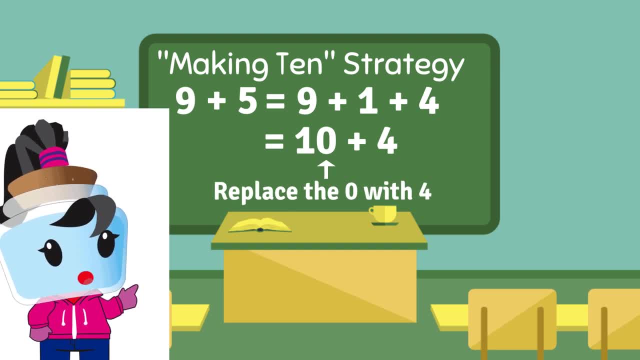 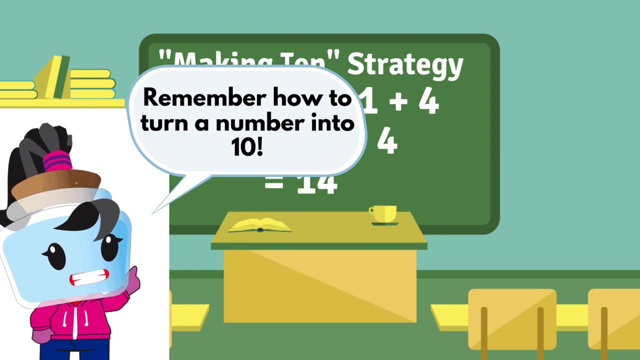 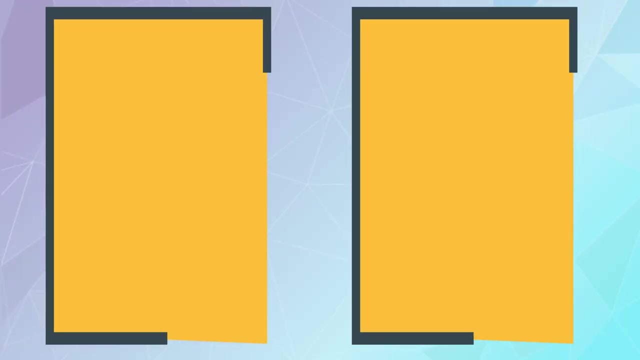 we simply replace the zero with the value. So now we have 10 plus 1 plus 4.. Now we have ten plus four equals fourteen. This trick is easy to use, as long as you can turn one of the values into ten. Let's practice this by solving these equations. 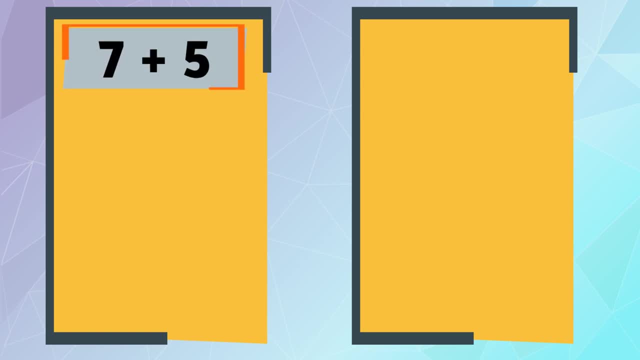 Seven plus five To make ten. we can take three from five and add it to seven. If we do that, we can rewrite the equation as seven plus three plus two. Seven plus three equals ten. So we can rewrite the equation again as ten plus two.